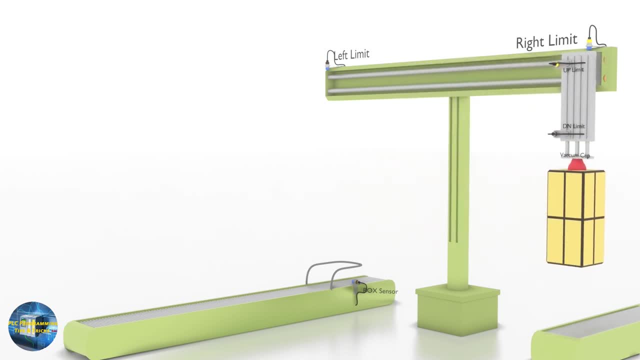 with the forward running three-phase motor and reaches the right limit sensor. Next the pickup cylinder moves down to the down limit sensor and turn off the vacuum output and drop box on the right side conveyor. Meanwhile the pickup cylinder moves up and as soon as it reaches, 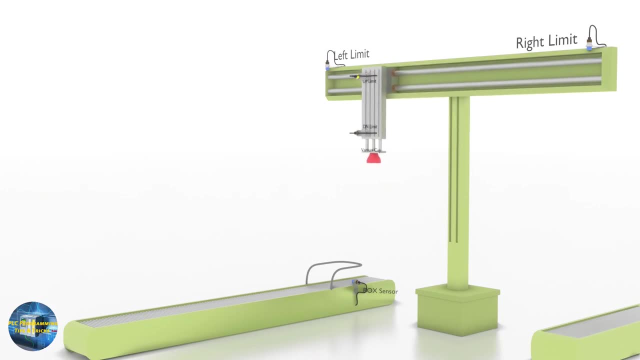 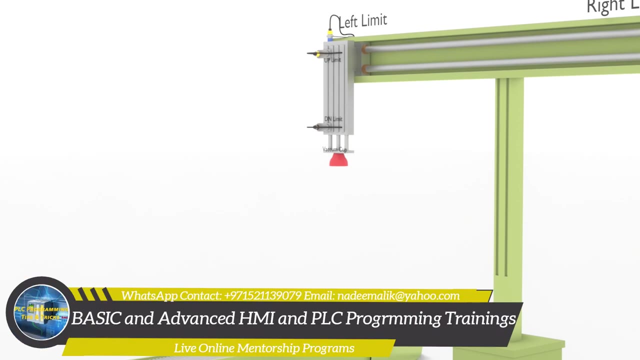 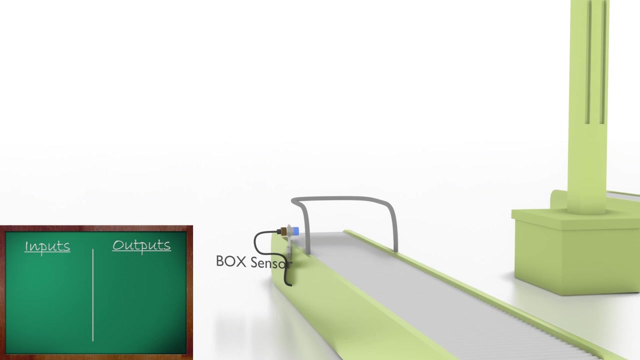 the up limit sensor. the whole system will travel toward the home or left side limit sensor and wait for the next box to come. Let's see closely the setup and discuss the addresses of these input sensors and outputs. First of all, we have a box sensor to detect the presence of the object. This sensor address is: 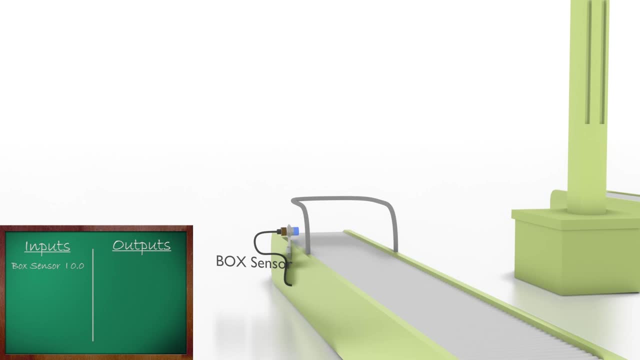 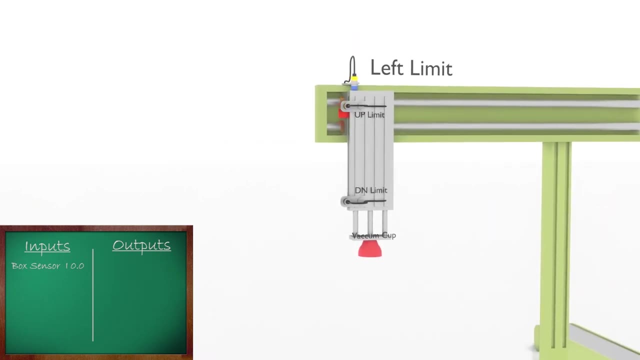 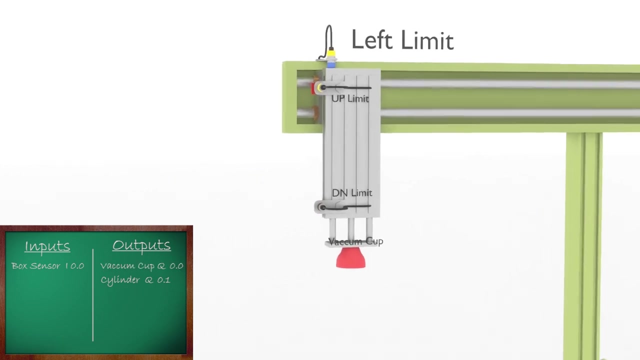 I0.0. Means. this sensor output wire is connected at I0.0 of the PLC. Next we have a pickup pneumatic cylinder which move up and down and create a vertical linear motion. This cylinder is activated by turning on the PLC output Q 0.1.. Next, a vacuum cup is attached in front of the pickup. 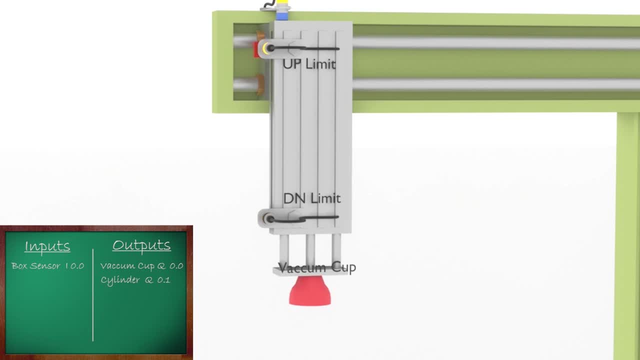 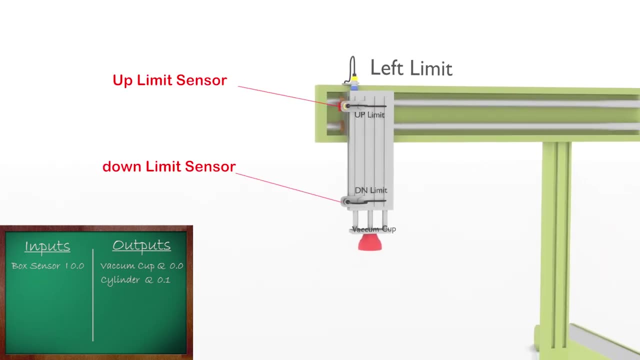 cylinder to grab the box. This vacuum cup is activated by the PLC output Q 0.0.. Next, we have two sensor to detect the pickup cylinder position. We have installed up limit sensor and down limit sensor connected at the PLC inputs I 0.1. 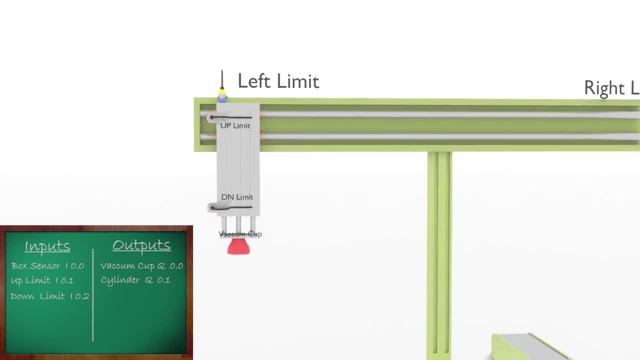 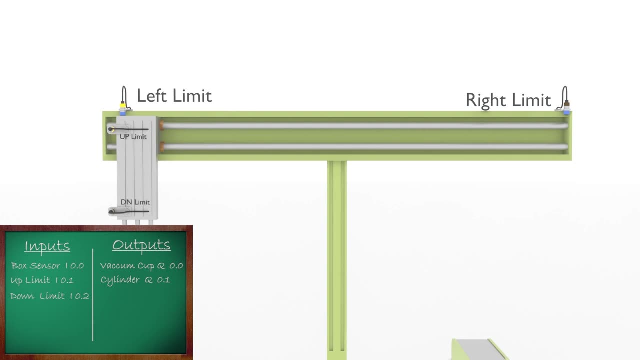 and I 0.2 respectively. Next, we have to move this whole set up to the right side. We have a three-phase motor to move the whole set up in reverse and forward direction. When we turn on Q 0.2 output of the PLC, it will energize the. 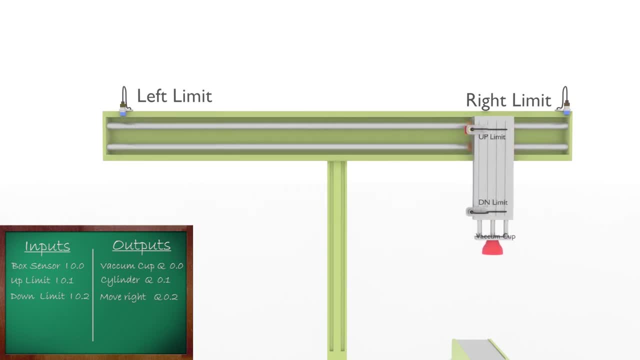 vacuum cup. Next it is switched OFF. Next we are turns on the AC Guy mode. Next we have a forward contactor and system will go to the right side. Next we have to bring the system back to the left side. We have to energize the reverse contactor by turning on the Q0.3 output of the PLC. 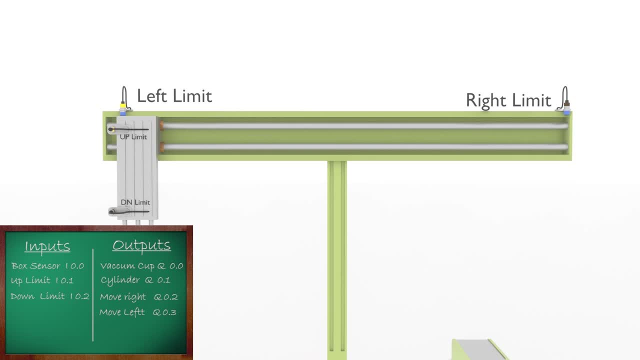 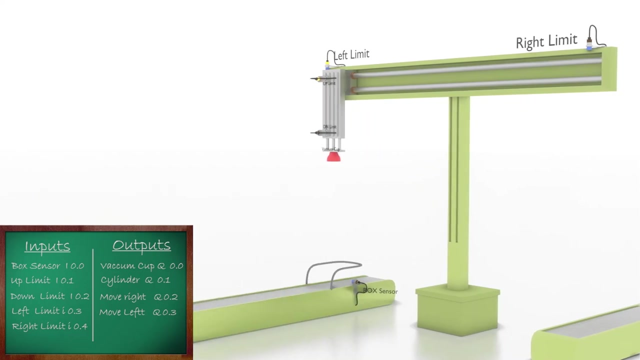 Next, we have installed two sensors to detect and confirm the position of the system on both left and right side. The left and right limit sensors are connected to I0.3 and I0.4 input of the PLC. These are the addresses of the inputs and outputs. 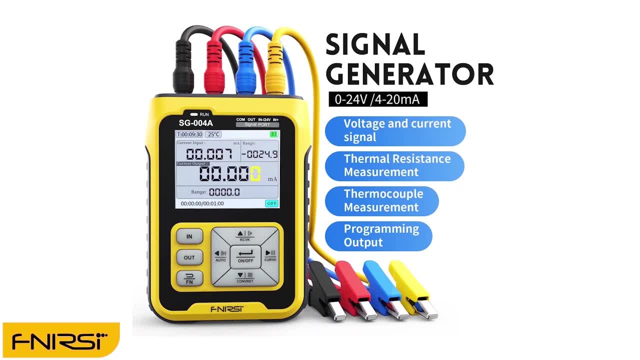 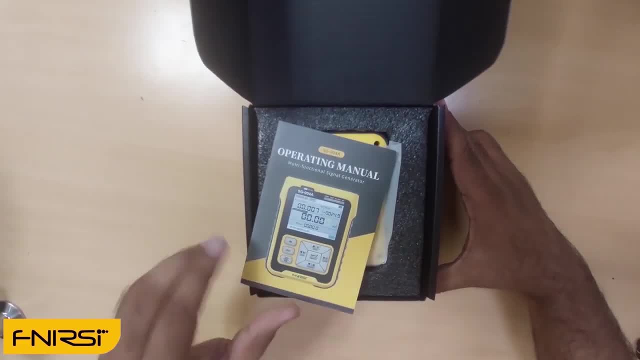 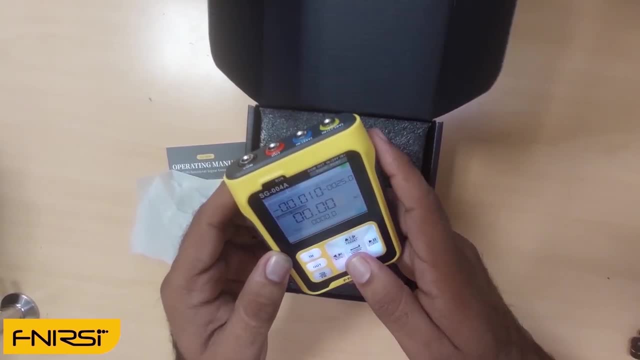 The I0.3 output is in kilohertz and we can also program output signal of this tool as per our requirement. Next, if we open this box, it comes in a very cool and secure packing. The signal generator tool feels and looks really cool. It is really handy and pocket size. Next, if we use the buttons, it feels. 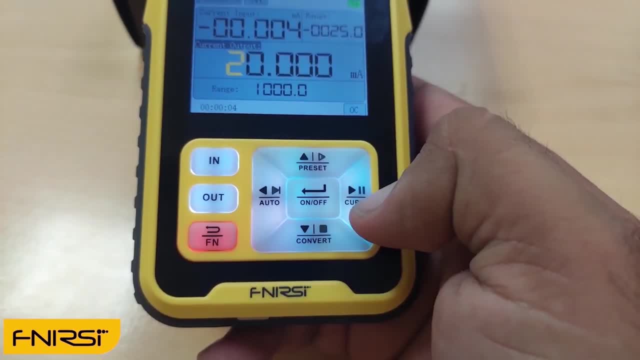 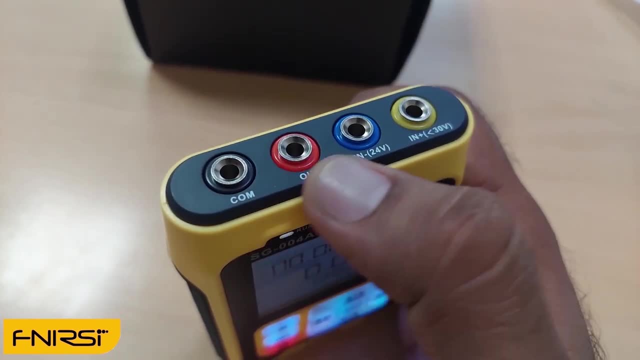 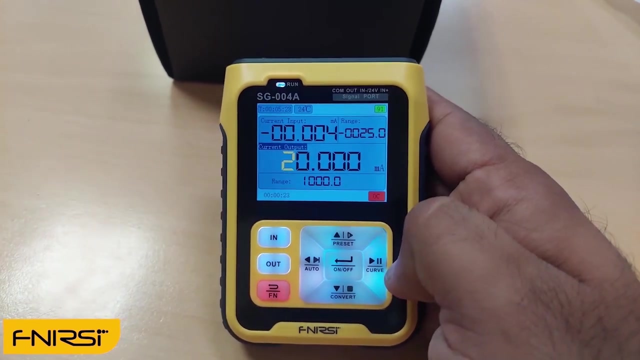 very tactile and the buttons are also illuminated with LEDs. Its build quality and plastic looks very robust and solid. These are the ports to connect the signal to the PLC. This meter is not only a signal generator, it can also measure world current frequency signals as well. Wire leads come with it. These also feel good. wires are soft and these crocodile clips. 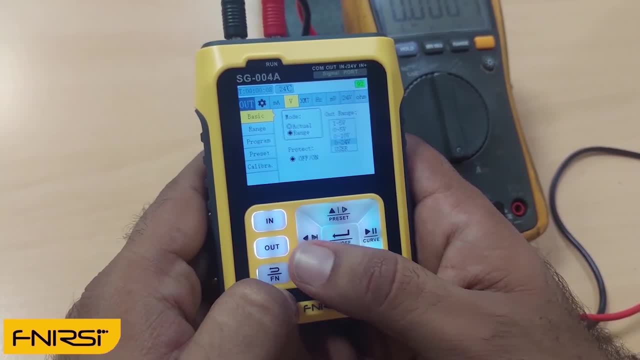 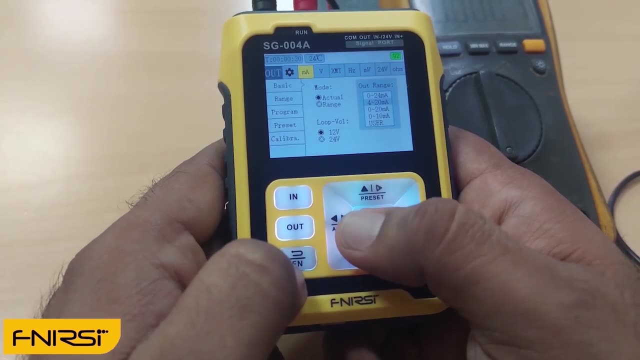 also feels good and robust. Let's test the signal generator and set the meter at 4-20 milliamps. signal generator. We will go to the input menu and set the current signal range at 4-20 milliamps. As you can see that our multimeter is right now showing. 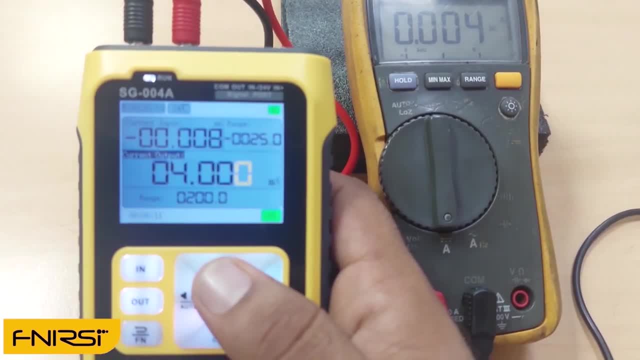 the future output signal range. This will show the current output signal range. If we increase this and increase it, then we will see this show the current and next we will see the current output signal range- 4 milliamp signals. and as we increase the signal from the tool multimeter also shows that this tool. 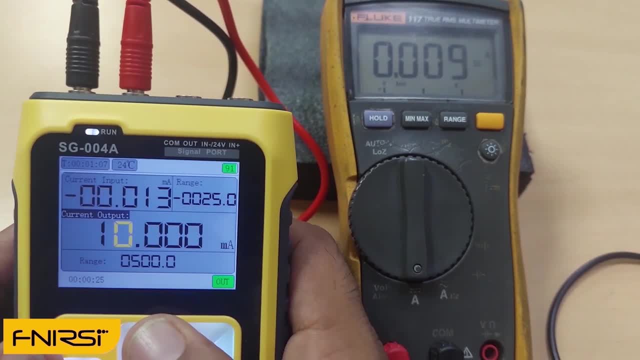 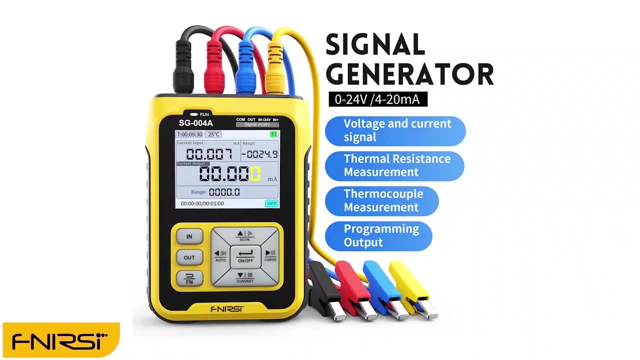 is really affordable, especially if you are beginner and want to learn, or you are expert and want to troubleshoot the analog signals. this tool is really very handy. if you want to buy this product- the link is in the description- there are some other more cheap and affordable signal generators. 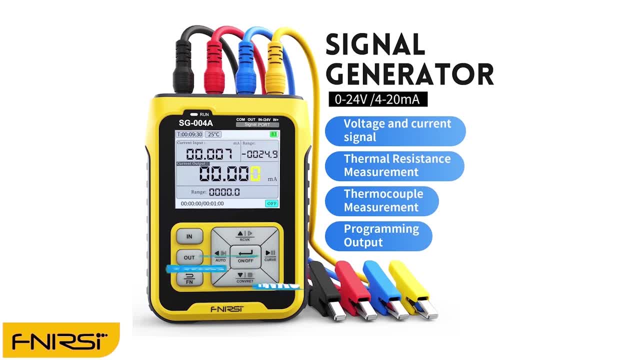 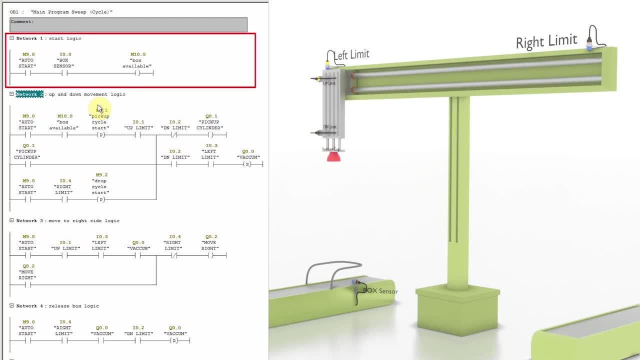 i have given the link in the description. just go to the video description and have a look on these as well. now let's see the ladder logic in network 1. we have a logic to start the process. it is simple logic. when the auto start, bit m9.0 is turned on and there is a box comes in front of. 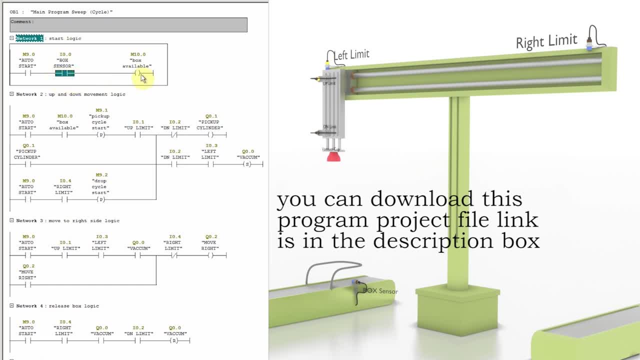 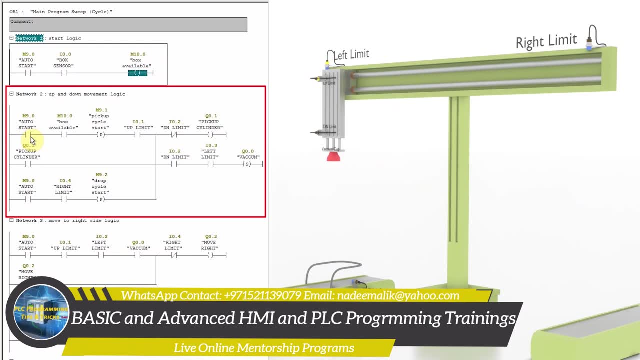 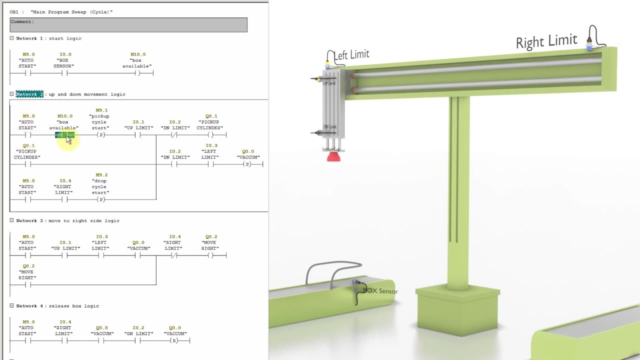 the sensor i0.0, it will turn on the box available bit m10.0. in network 2 we have written the ladder logic for up and down movement of the pickup cylinder q0.0. so when the auto bit is on and box is available on the rising edge it will latch on the cylinder bit. 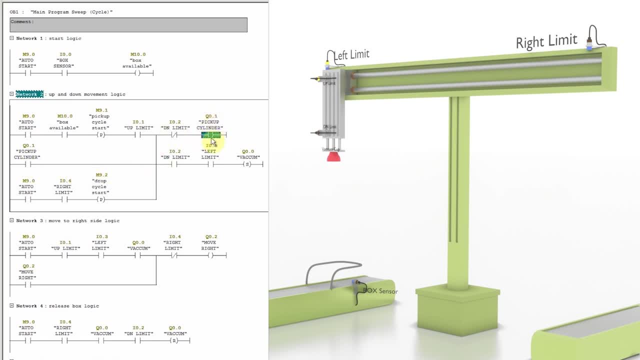 q0.1 and the cylinder will go down to pick up the box. this cylinder q0.1 will turn off when it reaches the down limit sensor i0.2 and cylinder will start to come back to its original up position. the second thing: when the cylinder reaches the down limit sensor i0.2, it is 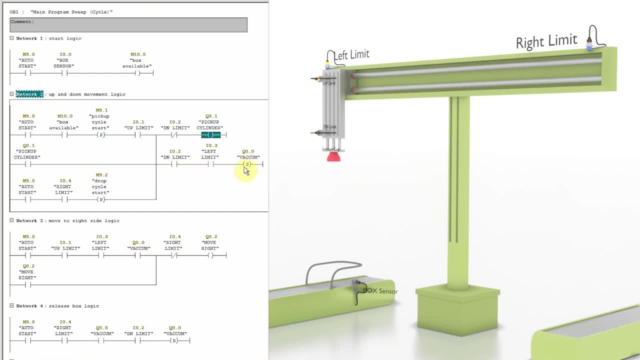 next to the box. it will latch on the system and push the button i0.3 to select the yourself load and speed. it will set the up of the cylinder to the right and wait at the left side. it will set on the vacuum output q0.0 to create a suction pressure to grab the box in network number three. 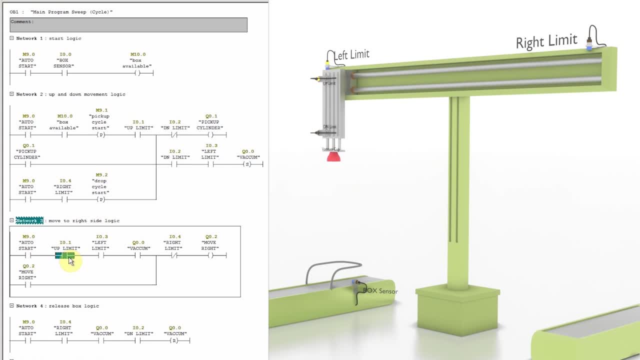 we have written the logic to move the box to the right side for this. the logic is simple: when the pickup cylinder is at up limit i0.1 and it is at the left side, confirmed by the sensor i0.3, and the vacuum output q0.0 is on, it will latch on the output q0.4 and vacuum output. 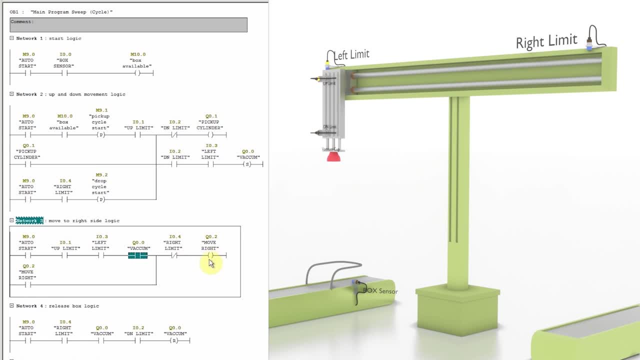 0.2 to move the system to the right side and this output q 0.2 will turn off when the system reaches the left side limit. sensor i: 0.4, as we have used the normal close contact of this sensor to unlatch. 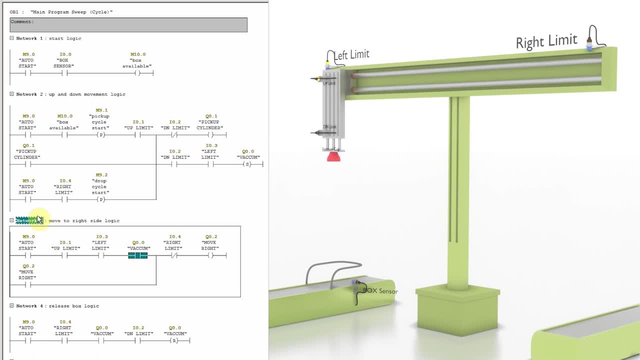 the output q 0.2. next, when the system reaches the right side position sensor i 0.4, it will turn on the pickup cylinder q 0.1 to go down and drop the box on the right side. when this cylinder goes down we have to turn off the vacuum output q 0.0 to release the box in the network. number four, when 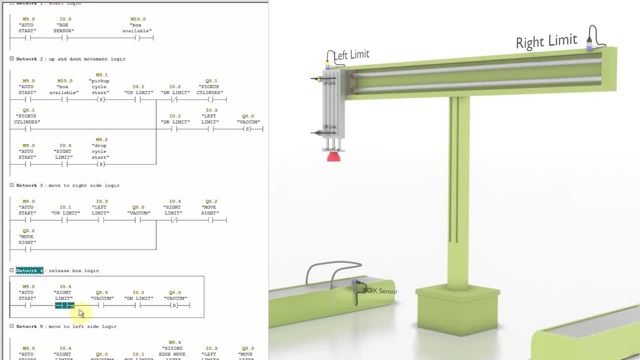 the auto bit is on and system is at right side, confirmed by the sensor i 0.4, and the cylinder position is down, confirmed by the sensor i 0.2. it will reset the vacuum output q 0.0 and the box will go down and drop the box on the right side. when the cylinder goes down, we have to turn. 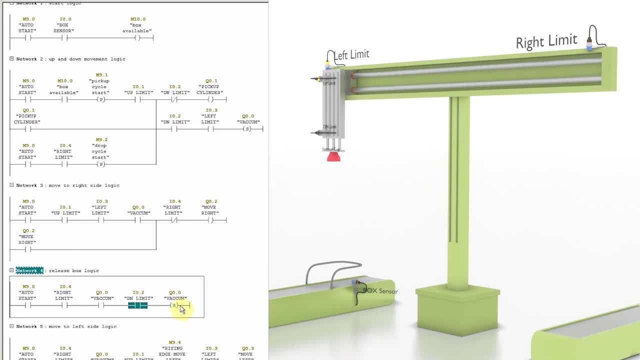 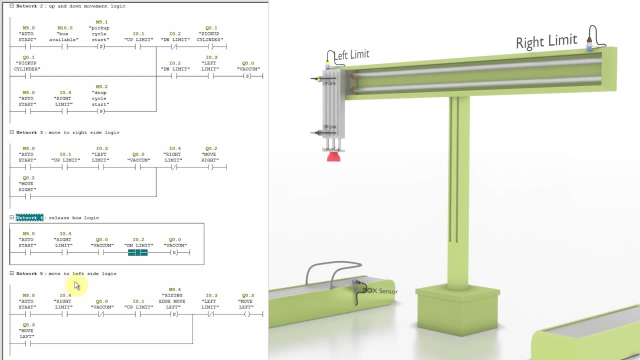 will be released on the right side conveyor. Next, after placing the box on the right side, the whole system have to come back to the home or the left side position In the network number 5, we have the logic to move the system from the right side to the left. 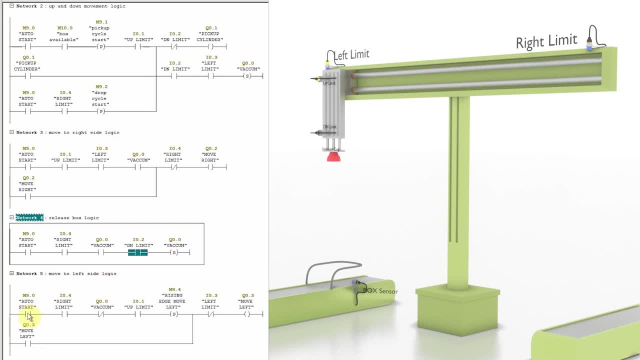 side home position. When the system is at the right side limit sensor I0.4 and the vacuum Q0.0 is off and the cylinder come back to the up limit sensor I0.1. on the rising edge of the RLO it will latch on the output Q0.3 to move the system to the left side by energizing the reverse 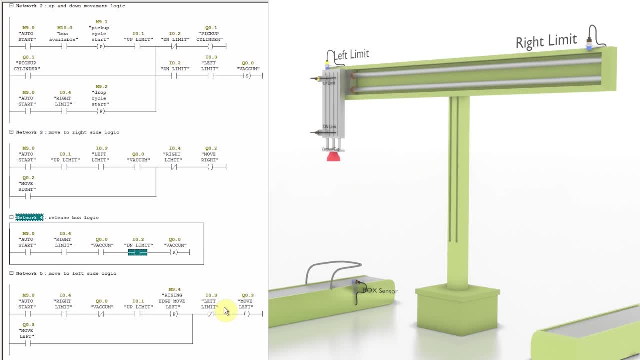 motor contactor. Once the system have reached the left position sensor I0.3,, it will unlatch the output Q0.3 and the system stops at the left side home position. So this is the program programming for the today's tutorial. next we will upload this program into the PLC and let's see. 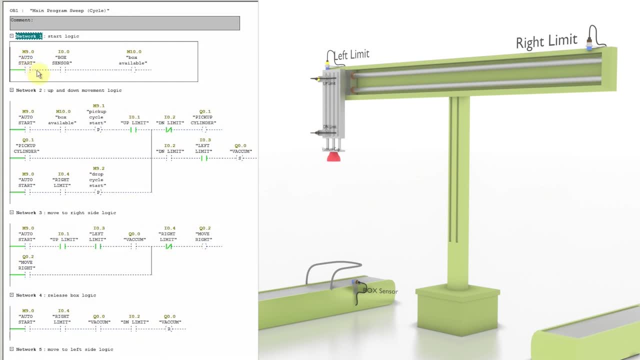 how does it works? as we turn on the auto start bit M9.0, the box comes in front of the sensor I0.0. it will turn on the box. available signal bit and pickup cylinder Q0.1 goes down, confirmed by the down limit sensor I0.2. it will turn on the vacuum output Q0.0 to grab the box and the cylinder. 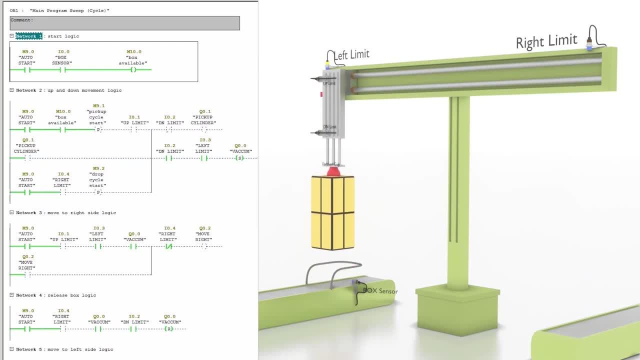 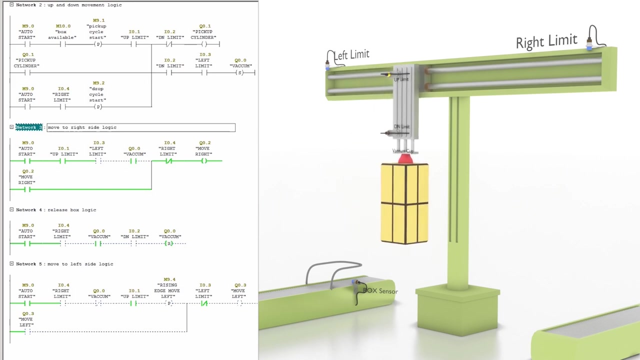 will move up to the sensor I0.1. now the cylinder is up and holding the box. next the whole system will move towards the right side limit sensor I0.4. as now the Q0.2 move right output is on, the system will stop at I0.4, right side limit sensor and the pickup cylinder Q0.1 again goes down to 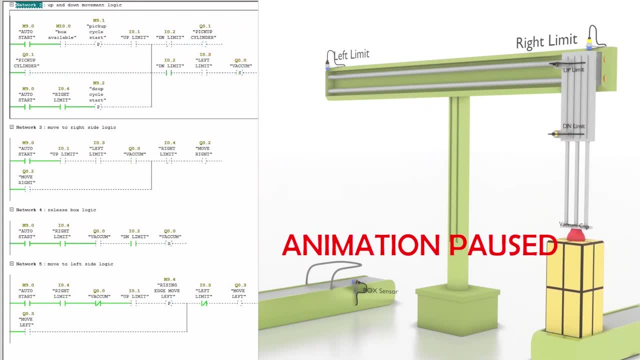 the down limit sensor I0.2. at down limit sensor position in the network 4, vacuum output Q0.0 is reset now and turned off and it will drop the box onto the conveyor. next the pickup cylinder. move to the uplimit sensor I0.1. 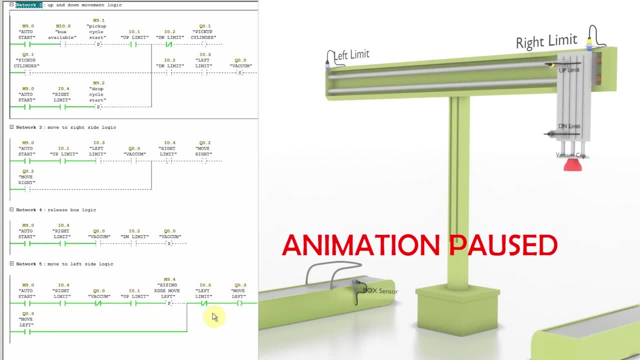 as soon as cylinder reaches the up sensor on the rising edge signal in the network number five, the move left output q 0.3 turns on and the whole system move towards the left side limit sensor i 0.3 and stops there waiting for the next box. so this is how we can make a program for this pick and place.